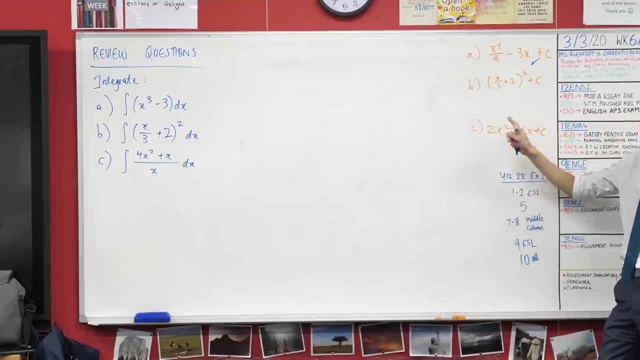 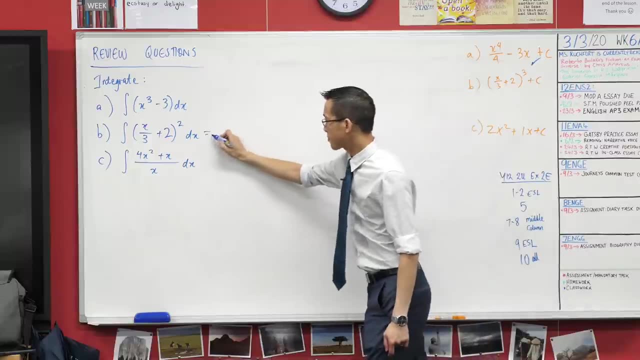 you either did that or came up with this answer. Let's have a think about how this came about, because this is the most efficient way I can tell. by the way it's written. okay, When we have a go at this. yes, we could expand, but if I can avoid it, I will, because expanding is a long process. 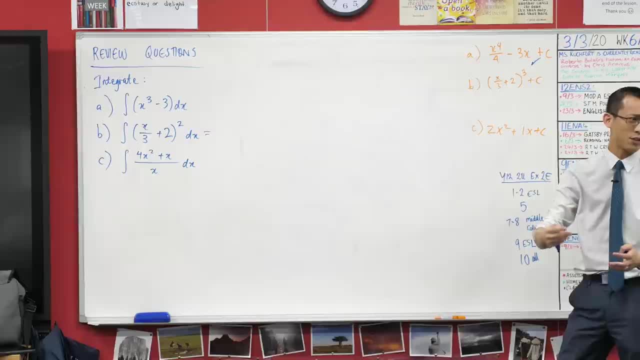 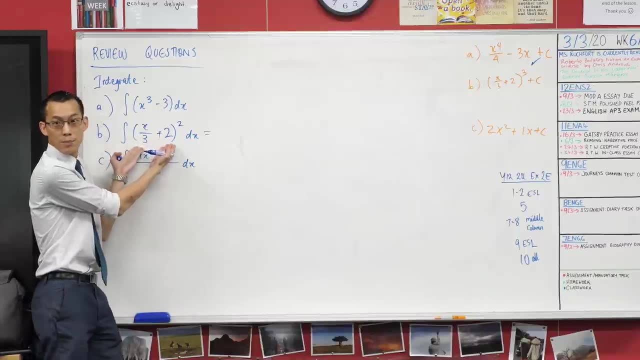 and then I have the have to begin integrating. so it's like two things that I have to do. I'd rather do just one. I can use the rule we developed a couple of lessons ago, which is the reverse chain rule. Here's a function and you're applying a different function to that, So I'm going. 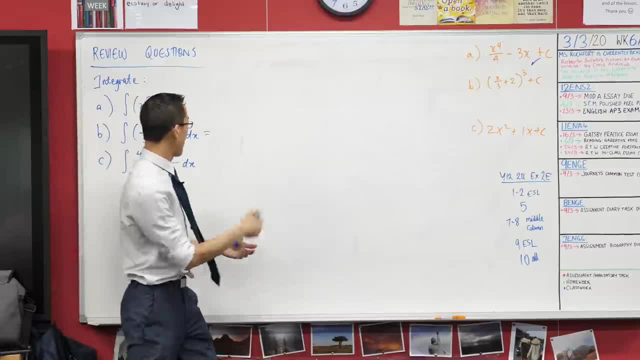 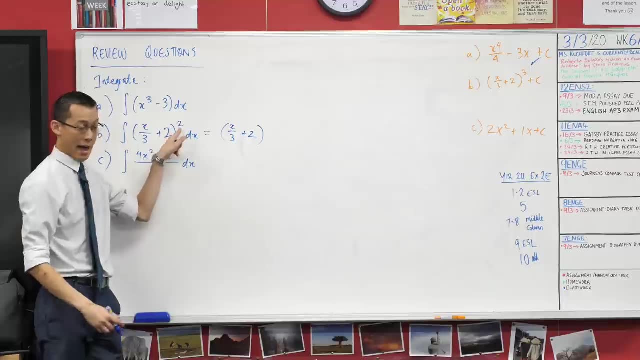 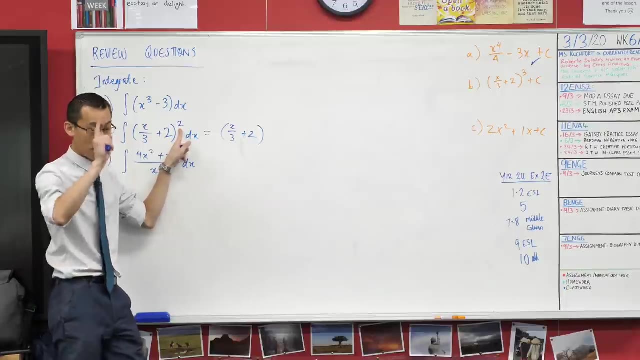 to try and undo reverse chain rule. Let's have a go at how he did it. You've got this x on 3 plus 2, and the power used to be 2.. When we're doing reverse chain rule, what happens to, I should say, index? The index goes to plus 1, so it's now a 3.. But then 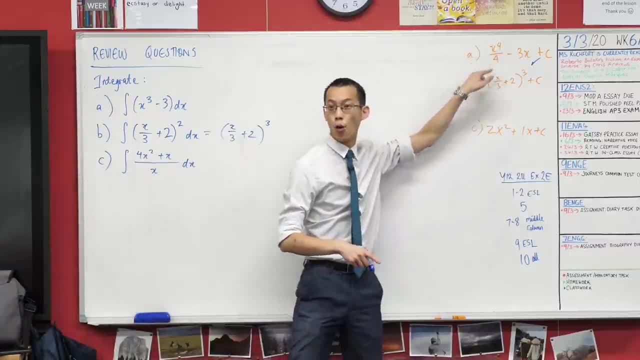 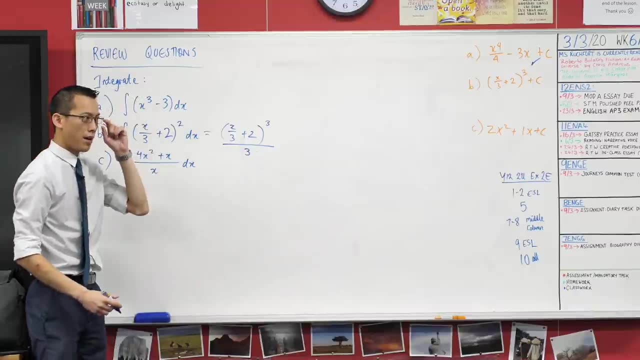 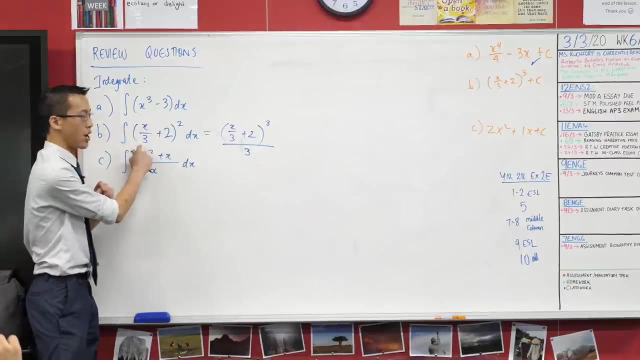 the next step is just like with this x to the 4 on 4, you divide by the new power, So then we get a 3.. Now, at this point here I've taken care of the outside, the squared bit, but I haven't taken care of the inside. The inside, the chain rule, rather does the 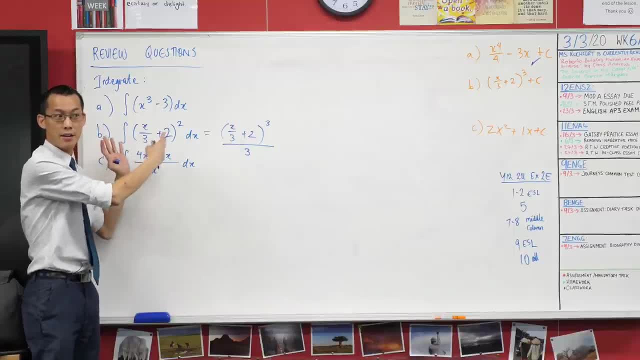 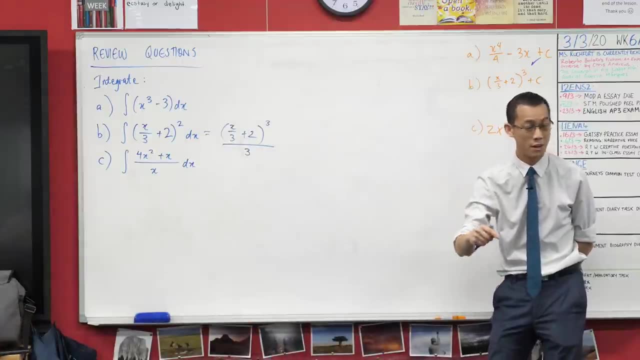 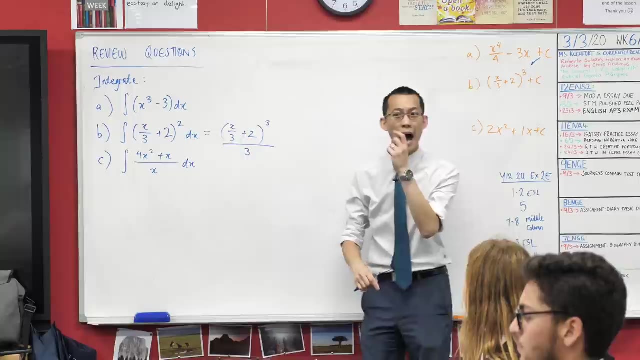 inside and the outside. The reverse chain rule also has to do the inside and the outside. What is the inside derivative? in this case, It's 1 over 3.. So this inside derivative, 1 over 3, what do I do with it? I divide by that. Now this is actually sneaky. A few of us have sort 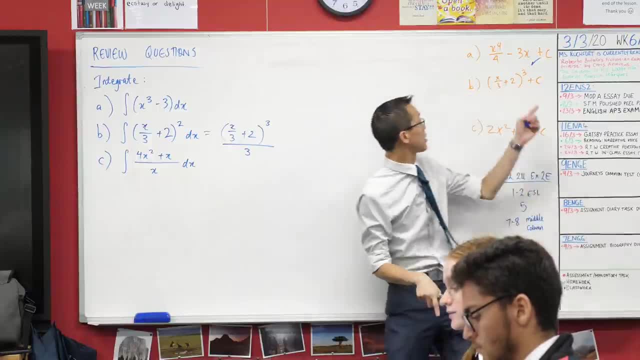 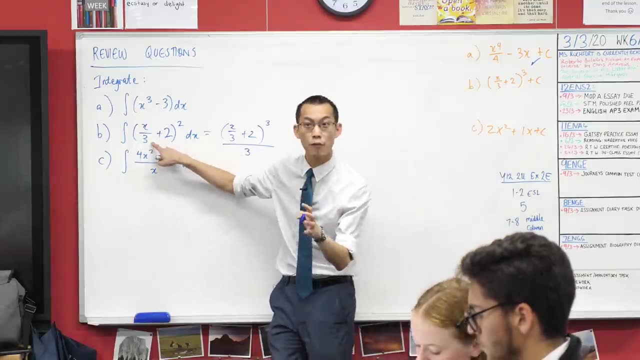 of been caught up, because when you integrate, you're going to get fractions. These kind of happen all the time And I've been, admittedly, mean to you by giving you a function, an integrand that will land. So I'm going to expand you with fractions on fractions, If you're dividing this thing. 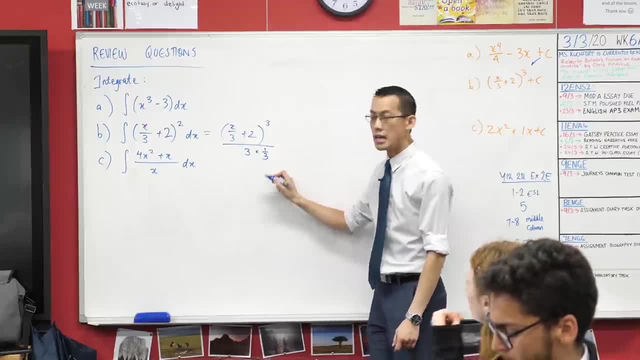 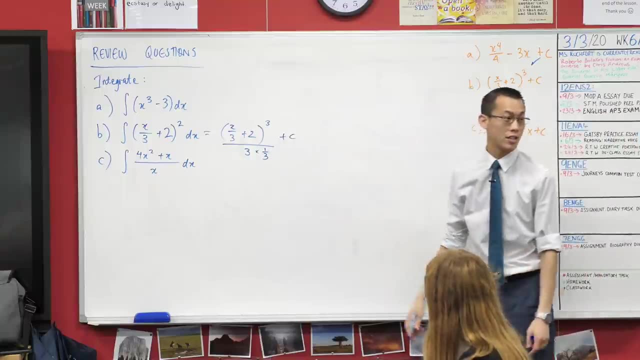 by a third, then the 1 third appears in the denominator, because the denominator is the thing doing division. So you can see here, once I add my constant of integration, which is always there, you can see how we get from here to the answer that Eddie's written Are. 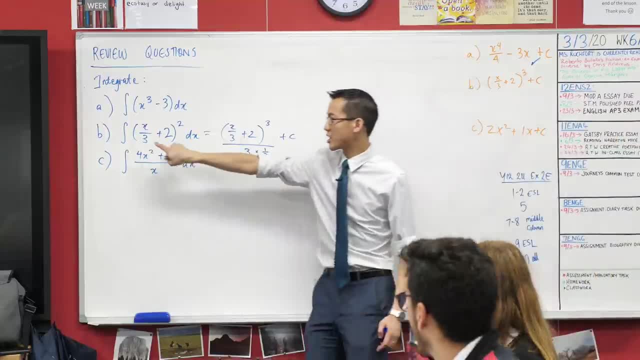 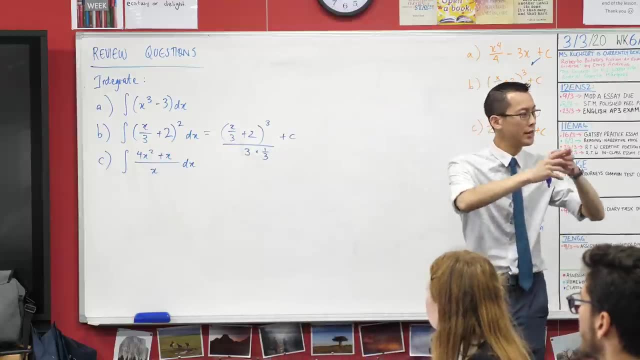 you happy with that. You can, of course, go ahead and expand all of this. provided you do the expansion correctly, You'll still end up with this, but it'll look different because probably yours will be in expanded form. This is factorized. 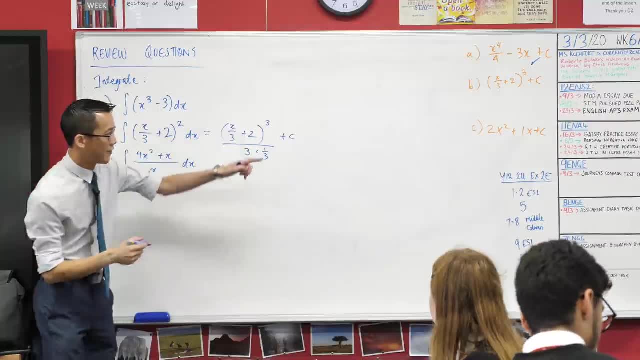 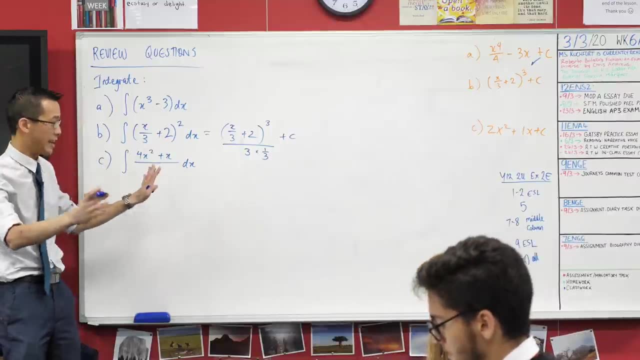 All right, last one Having a look at this answer here Was that you Moey. Yeah, That was your answer. Okay, Who's got that answer? A few, A few, Okay, just to quickly get how he did that. There's really one key thing you need. 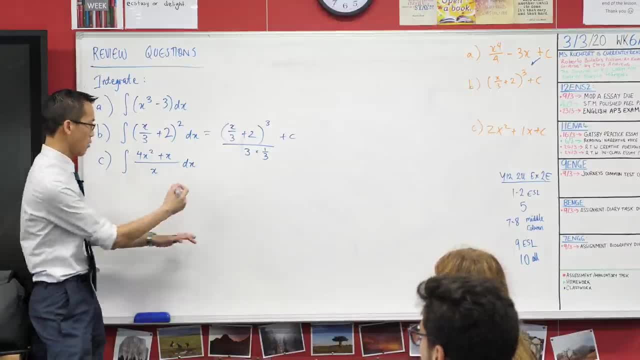 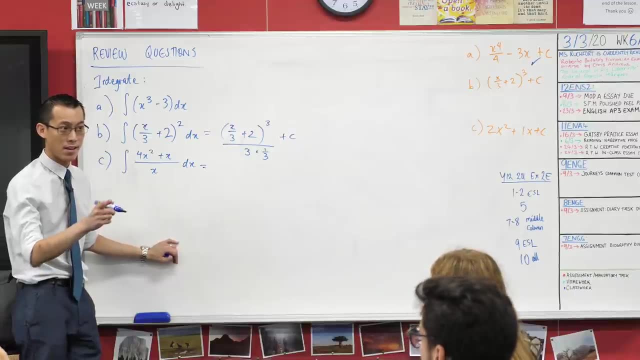 to do with this before you just proceed? as usual, We haven't been given the integrand in a nice form to work with. What should we do with it? 4x over h over x plus x over r. Okay, So we can take this part of the numerator divide through. separate it out: 4x squared. 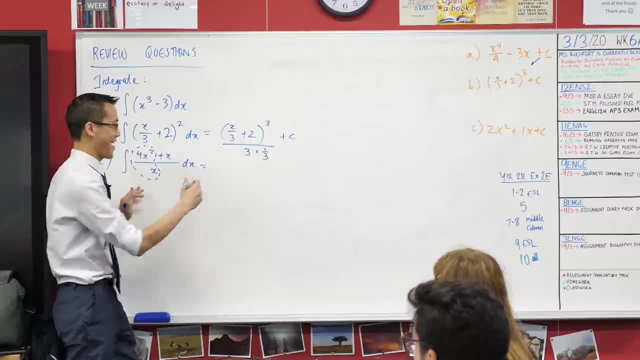 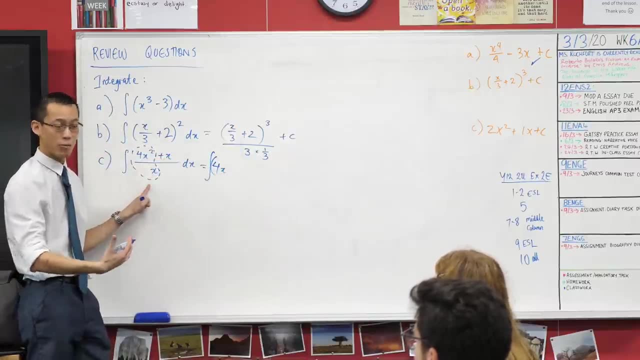 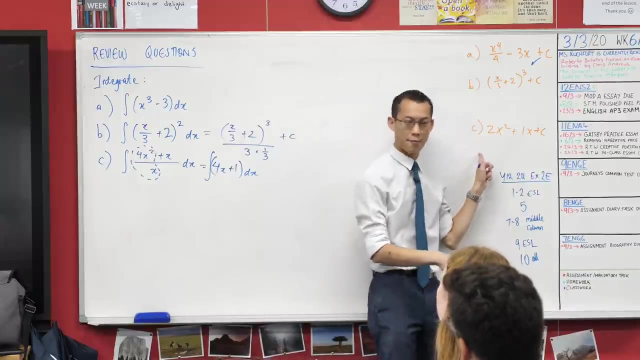 divided by x gives us 4x. Sorry, the integral sign is still there because I haven't done it yet. x divided by x. I can deal with that part, which is just 1.. And now that I've written it in a much neater form, hopefully it's now clear to you where this came from. The index. 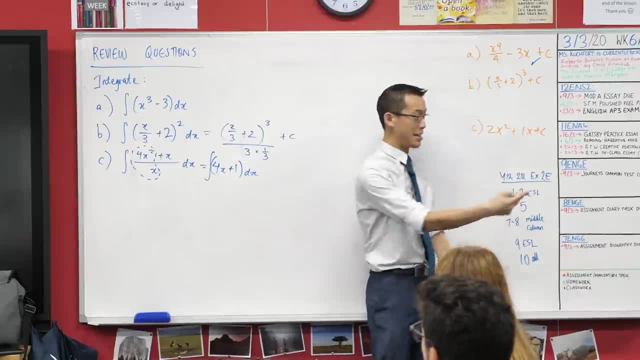 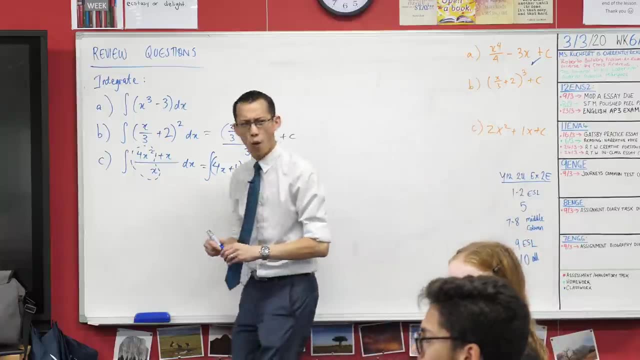 has gone up. He's divided by that new index. The 4 divided by the 2 leaves him with 2. And then off he goes from there. So thumbs up, Be happy. Okay, Well done, Okay, Well done. but we really need to work on affluency there. That took us way too long. 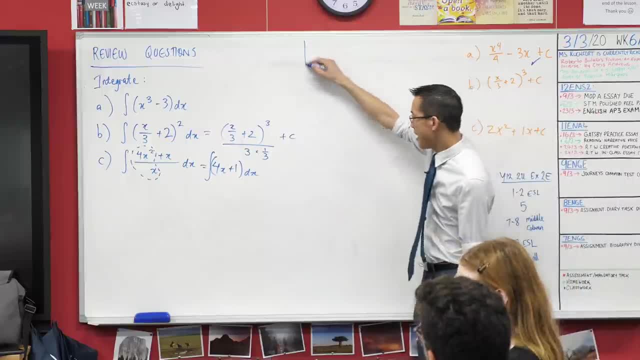 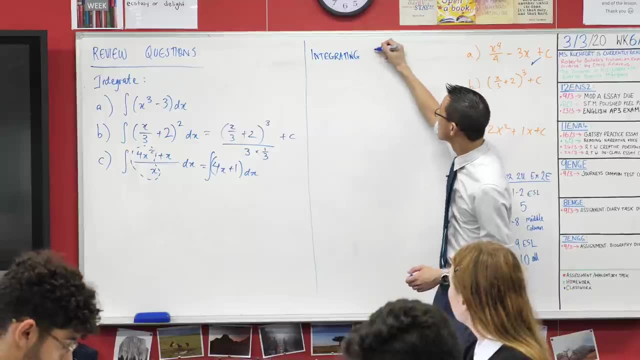 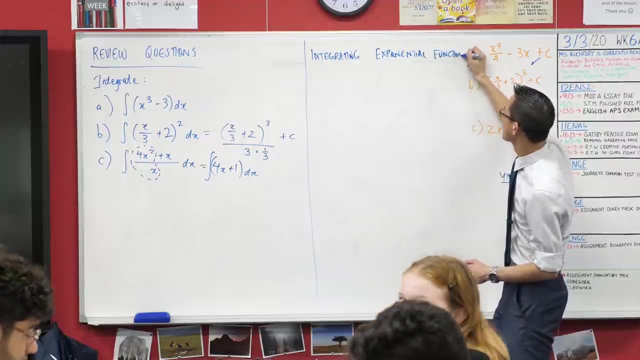 Okay. Can I ask you to rule that off and make a new heading which is integrating exponential functions? I was wrong, Though you could have been right. I mean, it was a good guess. It's a good guess, Okay Now. 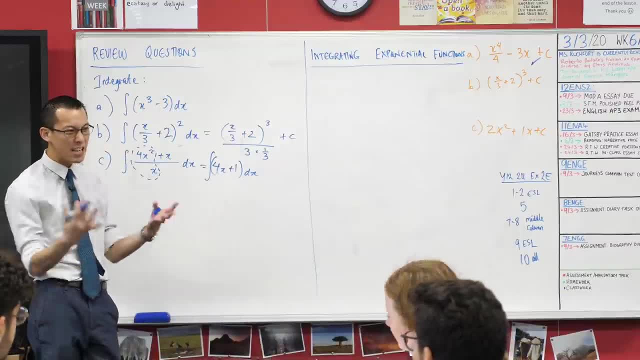 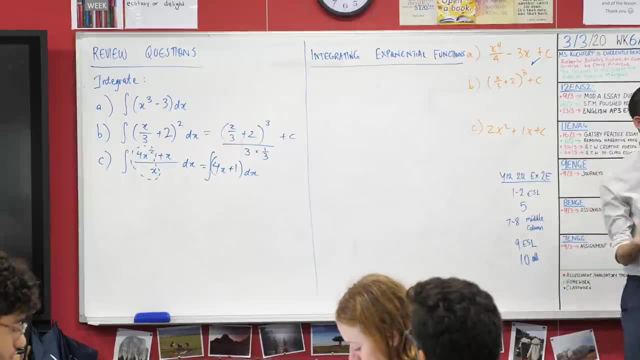 Now you will recall- we keep on saying it to try and drill it into your head- everything we know about integration, at least so far, everything we know about it we know from differentiation. We know how to differentiate exponential functions. In fact, they're delightfully 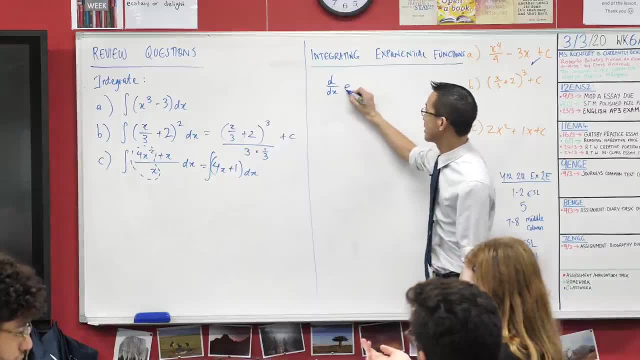 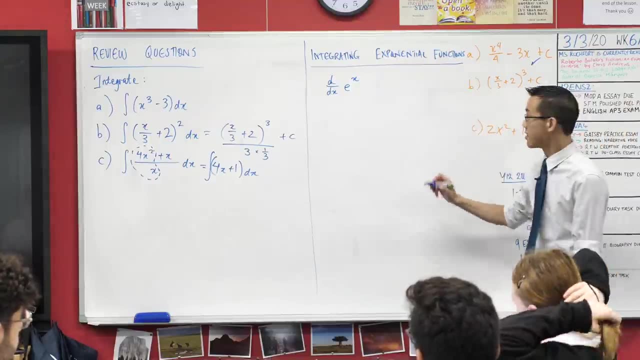 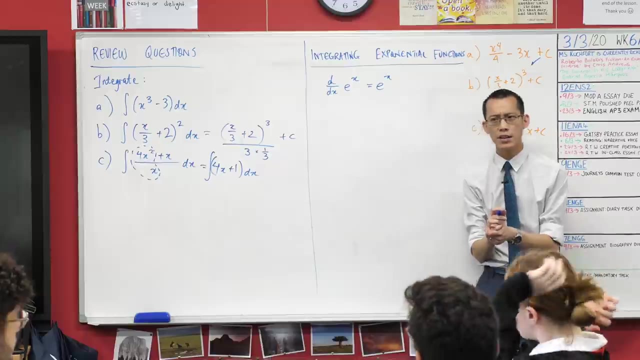 easy to differentiate, because if I gave you a function like, say this, you could say it's derivative, because you don't even, you almost have to do nothing. What is the derivative of this guy? It's e to the x. That's kind of the special thing about this specific exponential function. 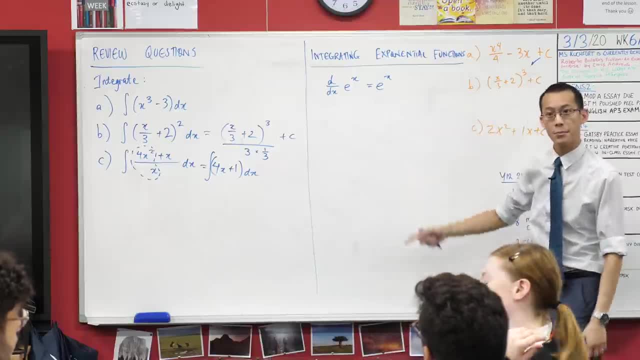 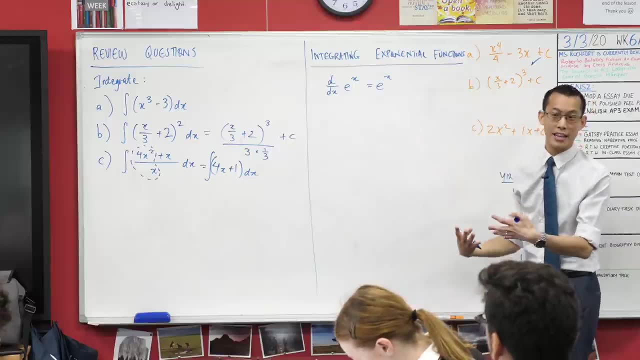 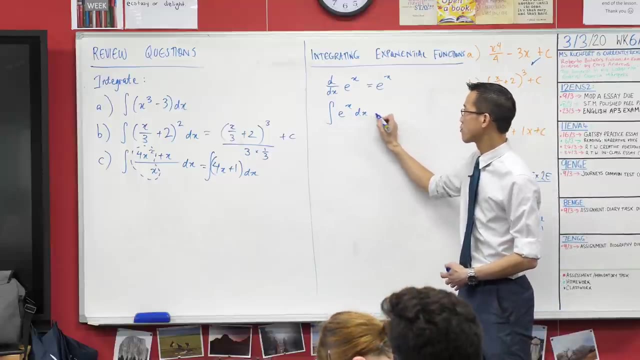 that when you differentiate it, you just get back itself. Okay, So since we have a statement about differentiation here, right, we can make an equivalent or parallel statement about integration. Yeah, What if I asked you to integrate e to the x with respect to x, What would you expect? 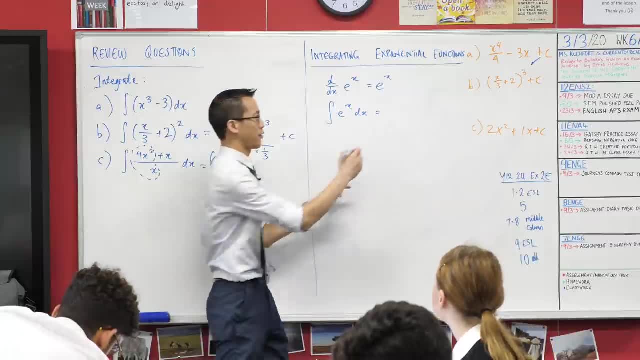 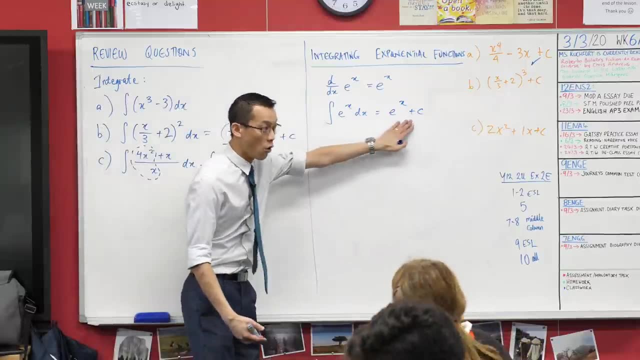 Yeah, So you would go back where you came from, with one subtle difference, which is that constant of integration, because e to the x plus 1, e to the x minus 500, they would all still differentiate and land us here, Okay. 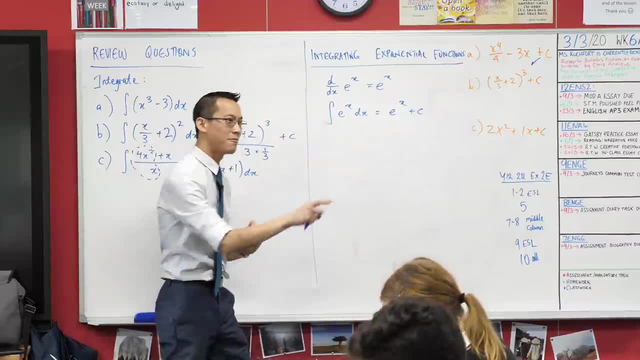 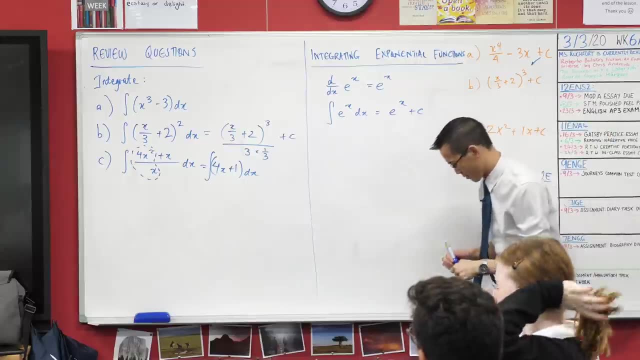 How about e to the x over x plus 1?? Ah, Can you say that again louder Serang? e to the x over x plus 1.. e to the x. I'm just going to write this down so I have it in my head. e to the x on did. 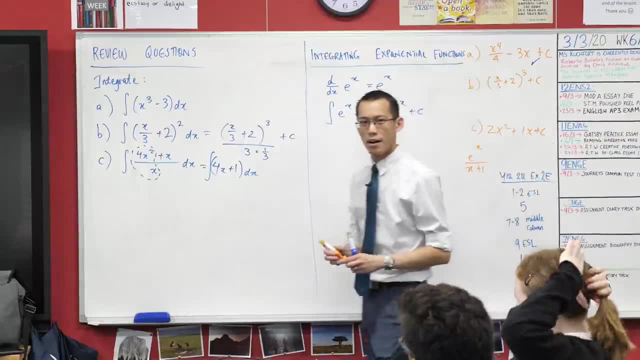 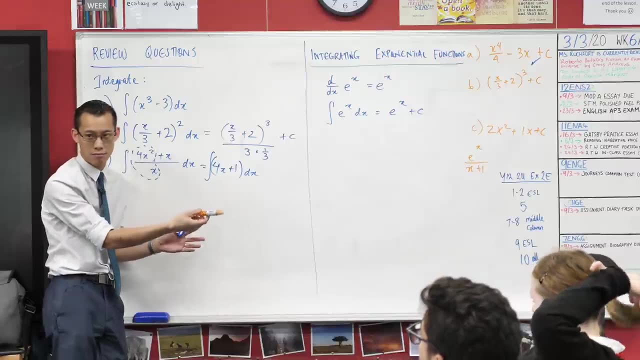 you say x plus 1? x plus 1.. Okay, I wasn't going to make this stop, but it's because it was mentioned. it's a good one. This is an error which crops up all the time. This is, in fact, not the integral, but it comes up frequently enough that it's worth. 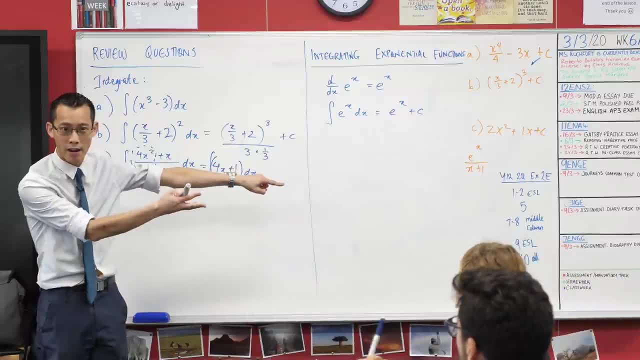 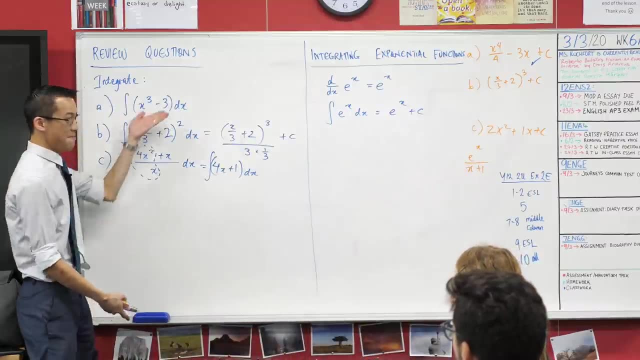 mentioning Where's this come from? by the way, This has not come from nowhere. Why might we think like? why are we in the habit of dividing? We've been doing that a lot, haven't we right? But why is that? 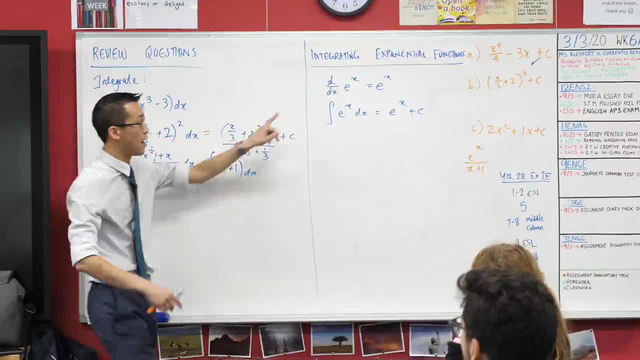 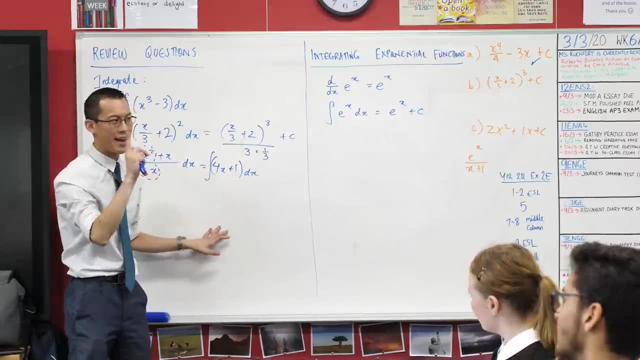 What kinds, what family of functions have we been dealing with so far? They're not exponentials. What would you call? all of these Starts with a p, We end up with- sorry, bad, yeah, I badly phrased the question. we end up with a primitive. 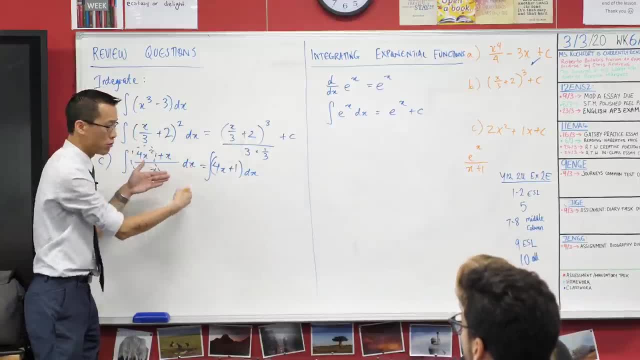 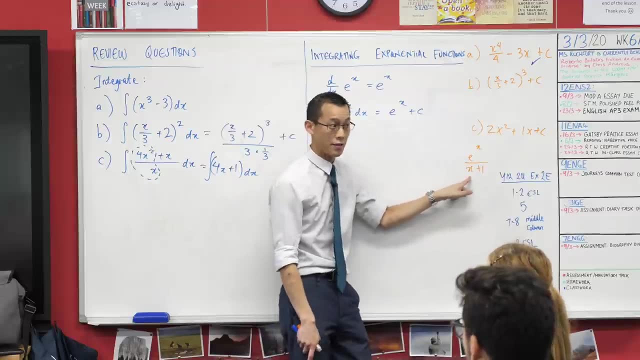 but what we were taking was a polynomial. the primitive ends up being a polynomial too. These are not polynomials, they're exponentials, so they behave quite differently. We don't, and you might have you know. another common error is that it's like increase. 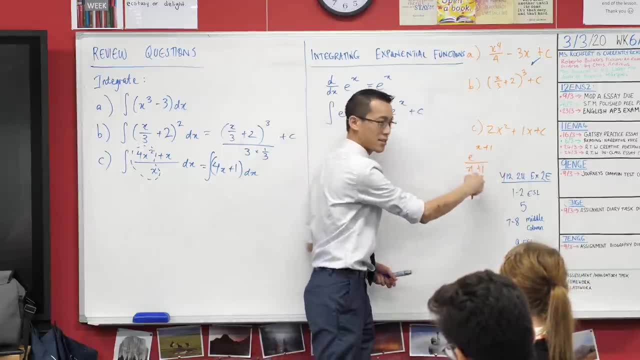 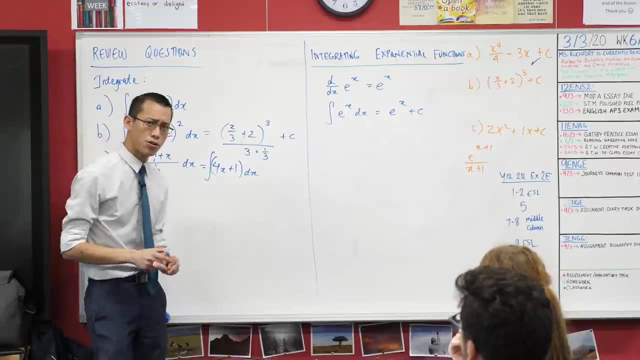 the index by 1 and then divide by that. but this is a whole different kettle of fish. okay, x is not in the base at all, it's in the index. okay, Let's see if we can push on this using, you know, this reverse chain rule stuff didn't. 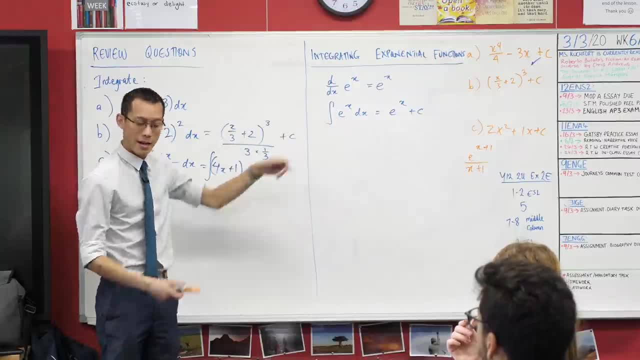 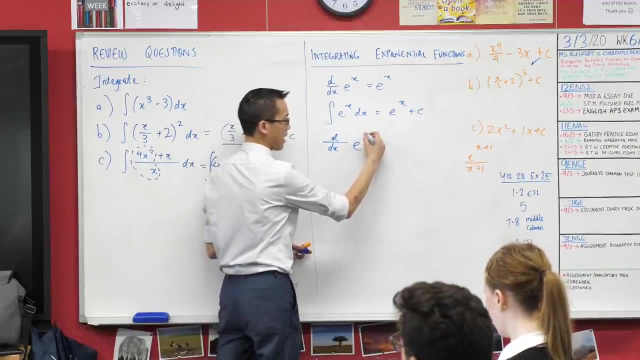 just apply to polynomials. it also applied to exponentials. So just to get your brain back in gear, if I asked you- and I'm going to ask you to do this right now- if I asked you to differentiate, say this: 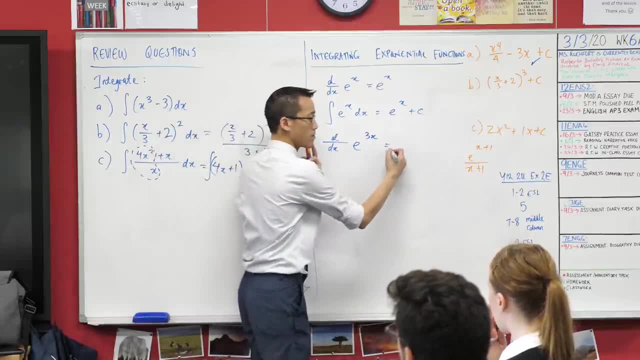 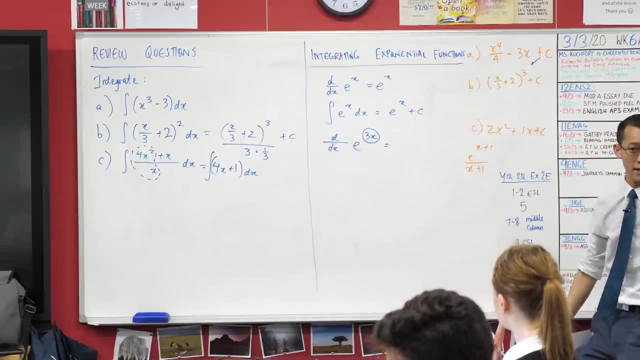 3e3x plus c. Okay, so you're doing again inside and outside. it's just: the inside is up there in the index, so its derivative, as Serene said, is 3,. okay, I've differentiated that part and now I do the outside. it's just an e to the power. 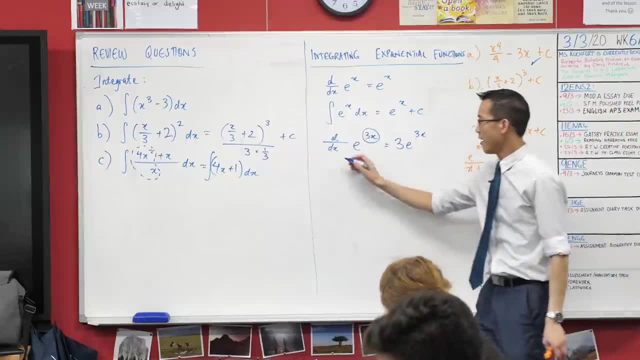 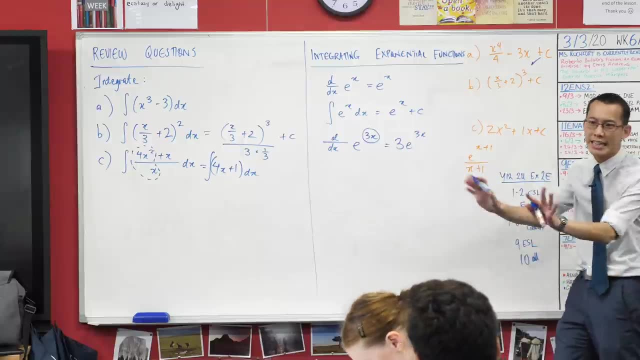 of it's an exponential. you just hand back that exponential Now, because on this line I've differentiated right. So is there any plus c? No, Not at this point We don't. we didn't need that for derivatives. 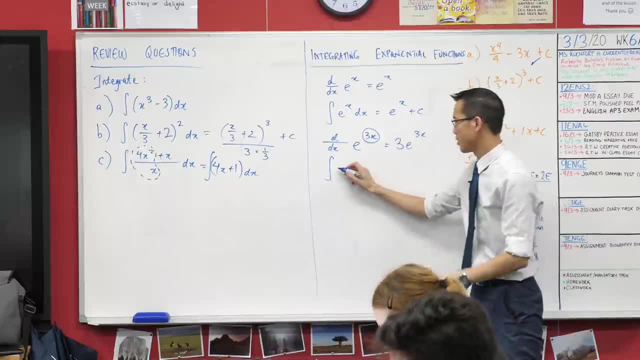 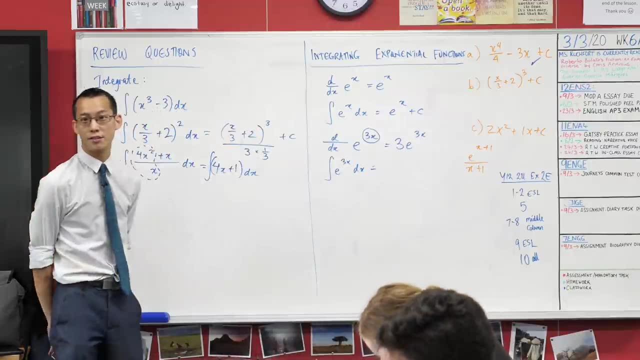 But now when I integrate, it'll be a different story, right? So now let's just take that same function, let's try integrating. We know integrating undoes everything that differentiation does. Here I multiply. I multiply by the inside derivative. 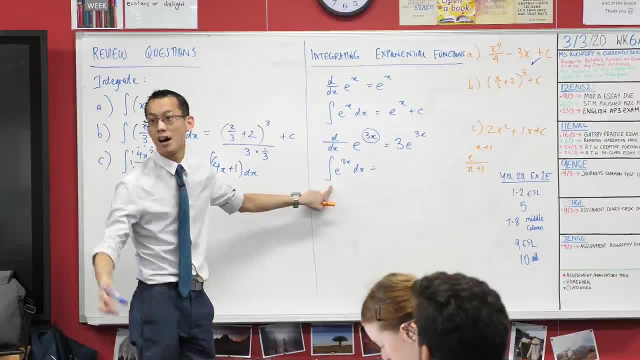 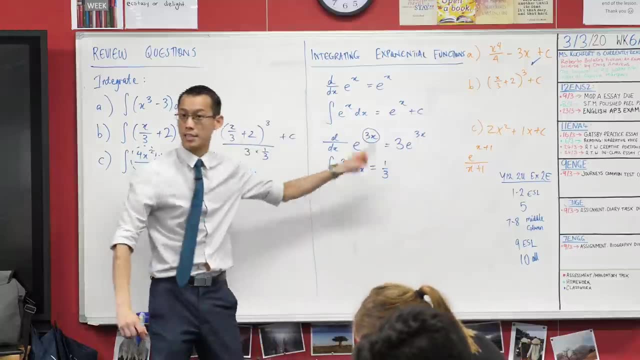 What do you think I should do here to undo that I should divide? Division's the opposite of multiplication. So I'm dividing by what? 3, so I'll just write a third out the front. that's me dividing by 3.. 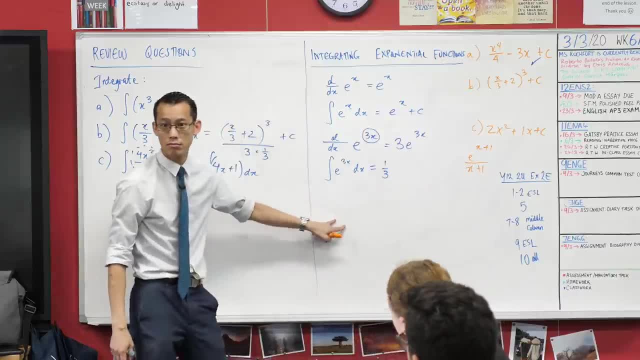 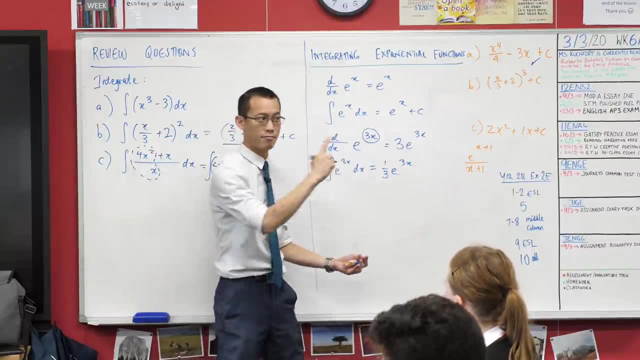 And then I've got to deal with this: what happens to that exponential? It just comes back to being itself, right? So it's e to the 3x. and now, because I'm integrating, constant integration, okay, And again, I implore you, a lot of you are asking me like. 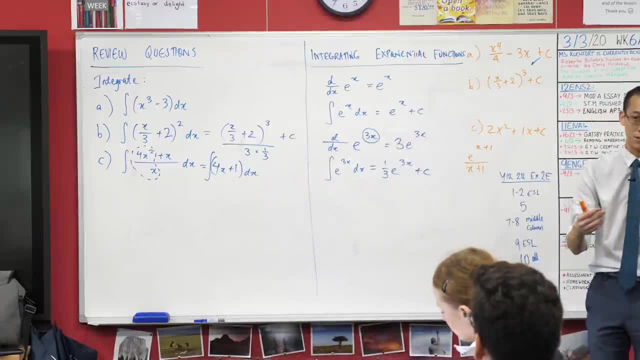 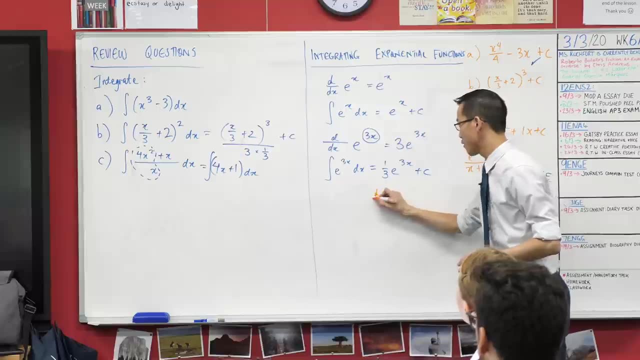 oh, have I got it right? okay, It's not just worth it- so you don't have to wait for a teacher to come around- but it's worth it for you to flex your differentiation muscles, to just have a look at this And say, if I differentiate this, am I going to bless you? 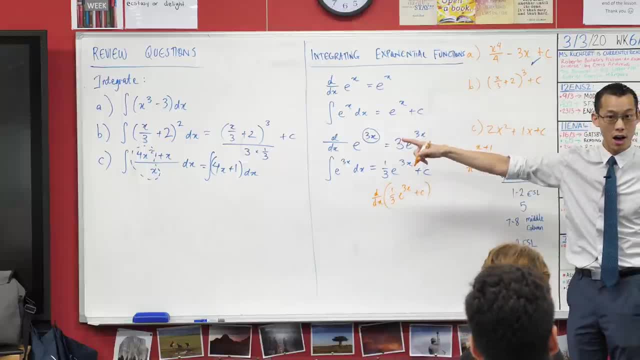 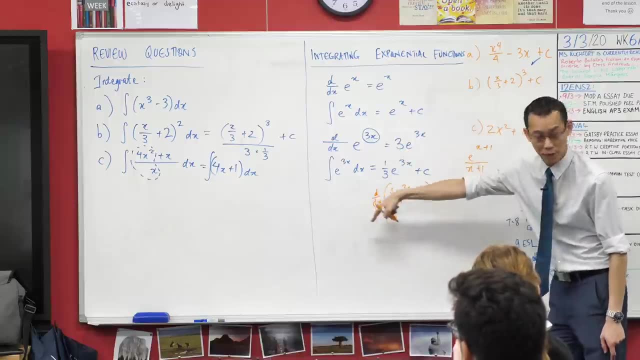 am I going to land back at the integrand I came from? What's going to happen? Yeah, that 3, just like here it's going to come out, the front 3.. The 1 third e to the 3x is still there. 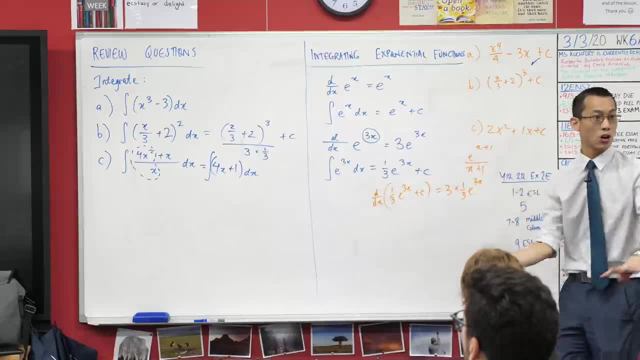 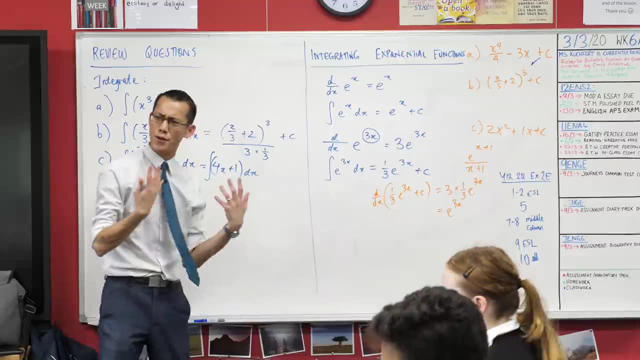 What happens? What happens to the plus c? It's gone. I can disregard it because it's constant. And there, thankfully, is what I was hoping for. This is just me proving to myself: oh yeah, I did get it right. because this is what I was supposed to integrate, okay.